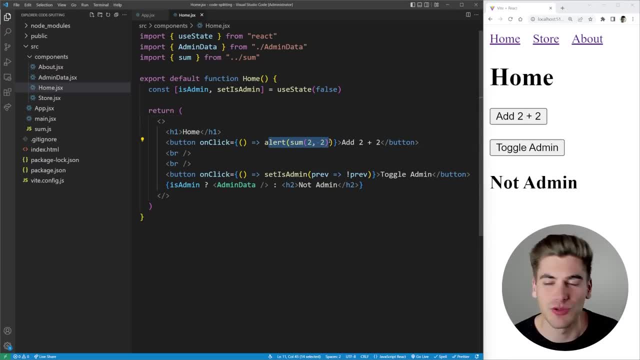 Also this sum function that I call right here to add the numbers two and two together. there's no point in me downloading that code until I actually click the button to add those numbers together. So the idea of code splitting is making sure you only download the code as soon as you. 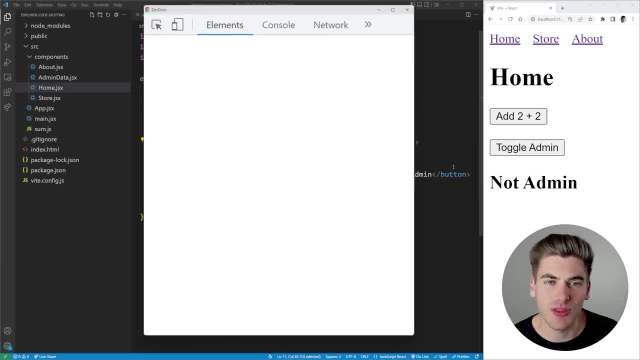 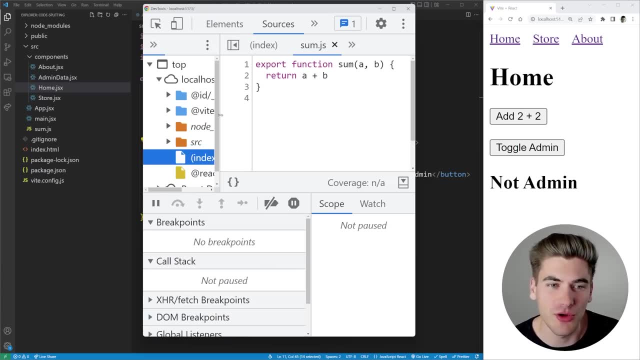 need it Now. if I just give the page a quick refresh and I just do an inspect on the page, this is going to be a fresh load of everything that gets downloaded as soon as I access this page, If I go to the sources tab, we can actually view all of the code that's being downloaded. 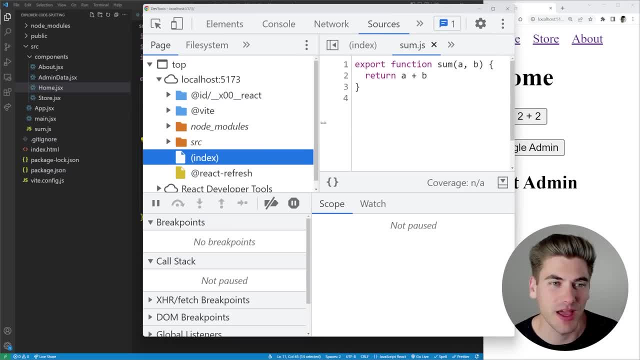 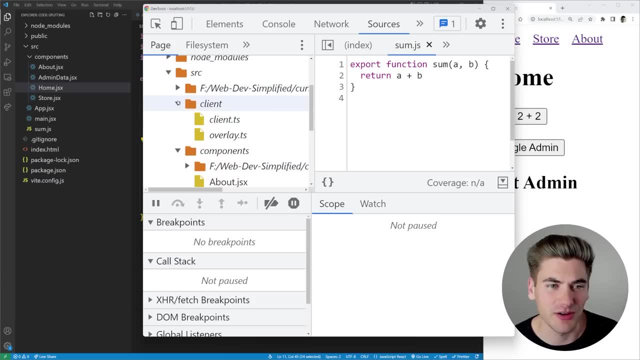 And the best thing that we can do is actually look over here on the left hand side where we have the file system. Essentially, if we go into this source folder you can see here we have our actual code and as well as our components folder and our client and 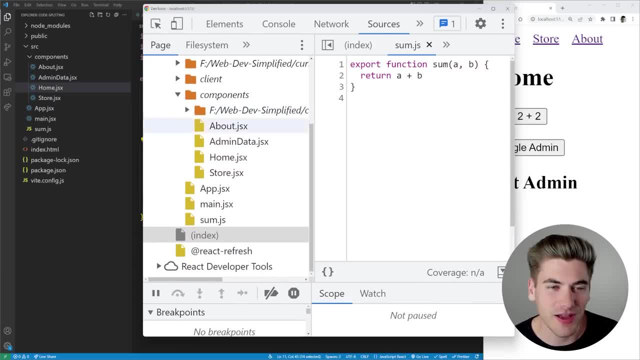 so on. But the main thing you'll notice is that inside of here, all of the files inside of our components being loaded. So if you look, here we have our about our admin data, our home, our store. we have here are some being downloaded, every single file in our project. 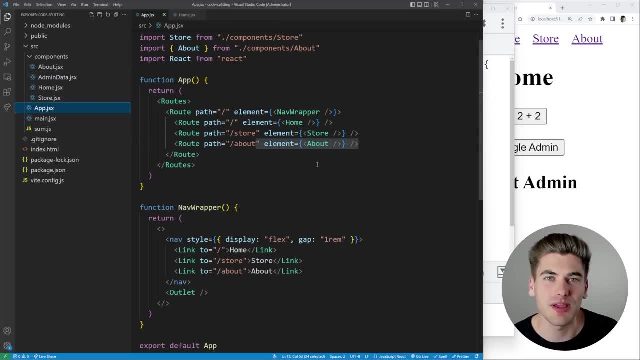 all of these files are being downloaded on the very first load of this page, While we're not actually accessing our store or about, so we should want to delay those files from being downloaded until we go to access those pages. This becomes especially useful when your project starts to get larger and larger, because if you download the entire file structure. 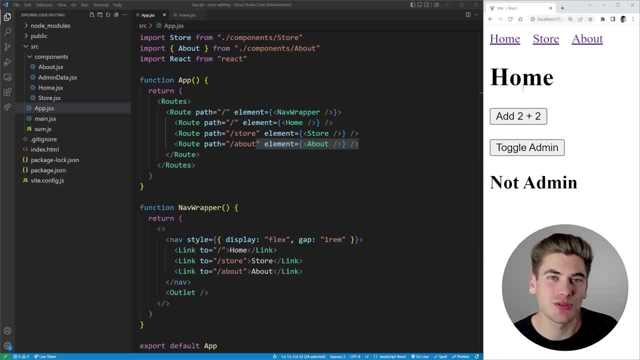 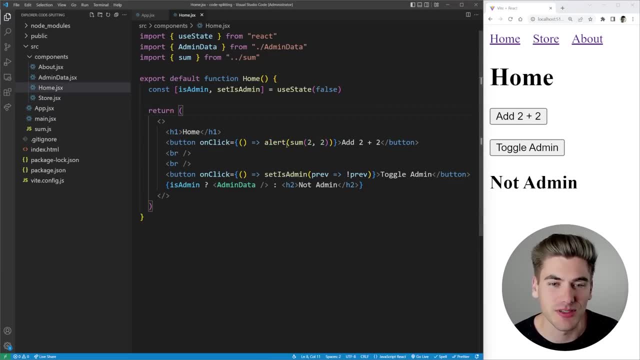 for the entire application at once. it's going to take a very long time, So splitting that up is going to be very beneficial. So the easiest way to do code splitting is if you just want to code split out a simple function, for example this: some function right here. I'm going to show you. 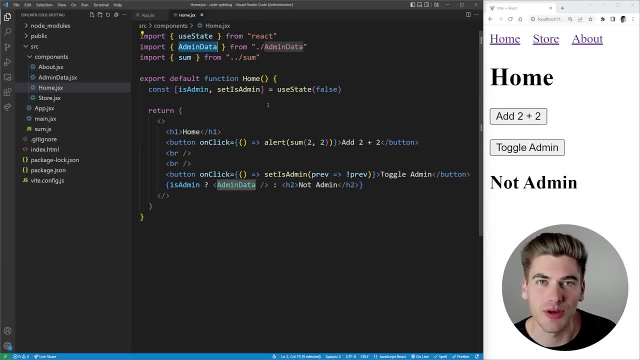 first how to do that And then I'll show you how to code split out individual components. So in order to code split something, we can use a dynamic import, And a dynamic import is going to only import the code when we actually use it on the page. So, for example, here instead. 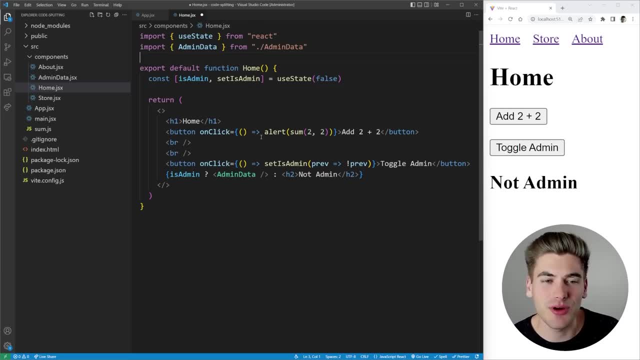 of importing my some function up here. I'm going to remove that import And instead I'm going to import it right here whenever I click on the button. So let's just put this on another line So it's a little bit easier to read. And what I want to do is I want to use import, but I'm going 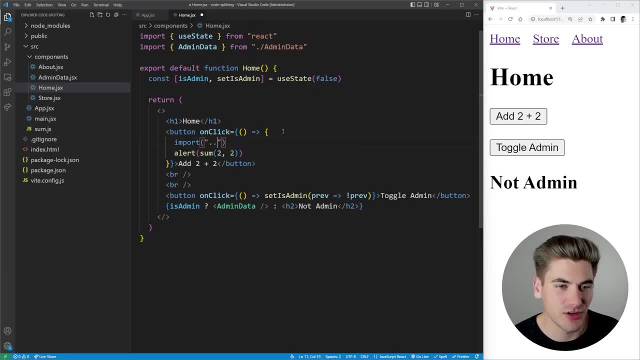 to call it as a function. I want to pass it the path to that file. So in our case it's just dot, dot slash, some just like that, And we'll just put the dot j s at the end there. So then, what we can. 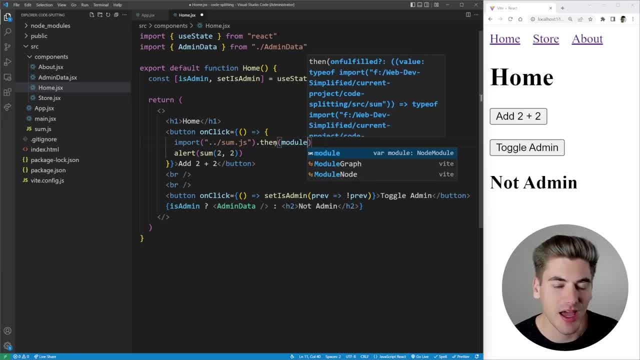 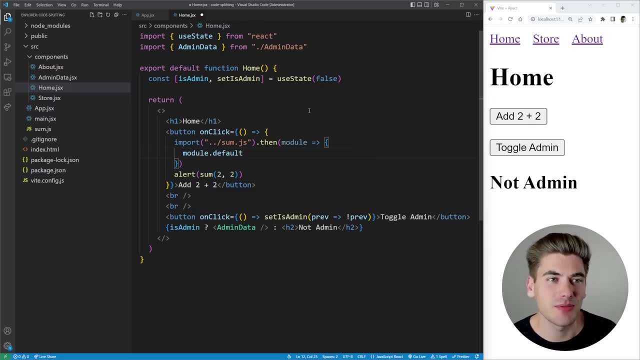 do is we can just say dot. then this returns to us a promise And that promise is going to have our module object inside of it. This module object is going to have a bunch of different properties, So, default, that's going to be the default export In our case. this sum is not a default export. 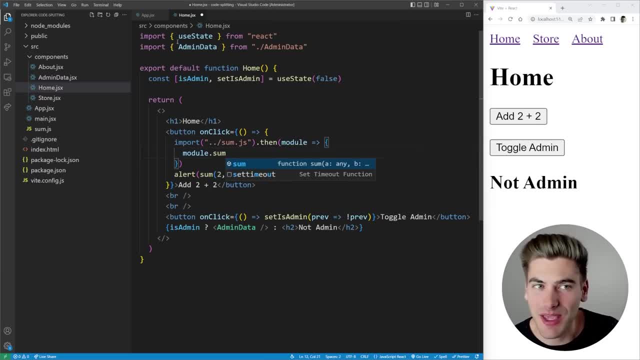 So we can say module dot sum And that's going to access the named export which we called some. if we had another export called like two, that is going to be just accessed like this. So we can say dot sum, we can put our numbers two and two in there. And if we just do a simple alert where 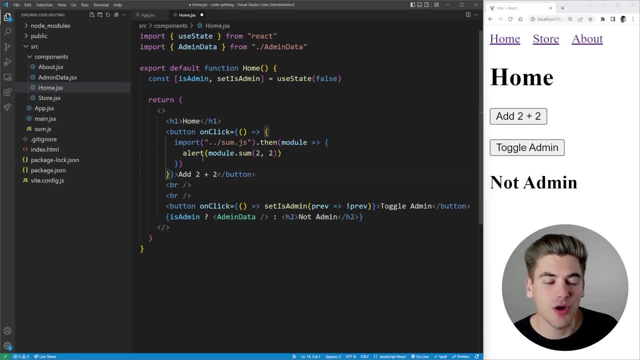 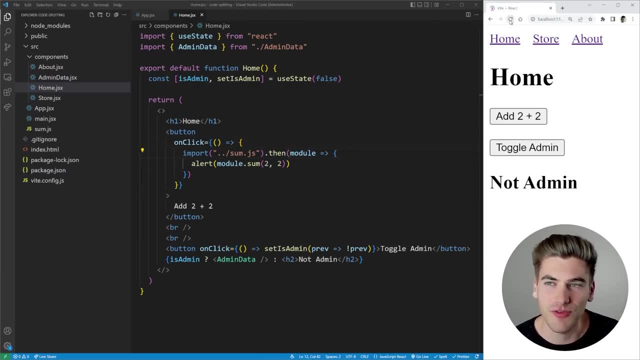 we are learning that out, so it works just like it was before. Now, when we click on our button, it's going to download the file for our sumjs And it's going to alert out that value. So let's do a really quick example of that, If I refresh. 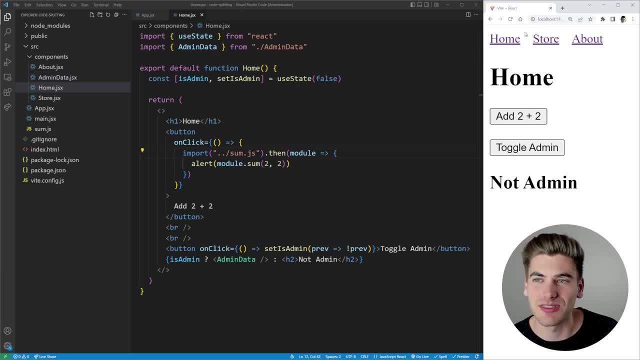 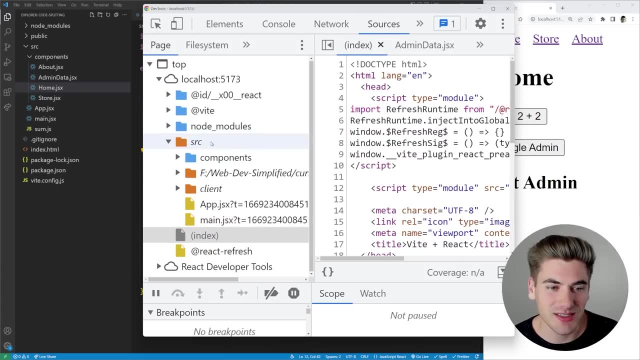 my page and I click the sum button, you can see everything works exactly the same as before. Let's do another refresh So we have a completely fresh load of our application. If I go over to that sources tab, you'll notice inside of here our sumjs file is not actually. 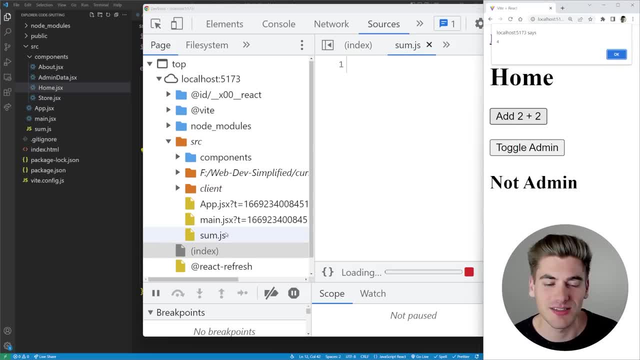 loaded yet. But as soon as I click on that button you'll notice over here on the left hand side of my screen that sumjs file has been downloaded onto the page and is actually running to do that summing. So it's not actually running or downloading that code until I actually need it. 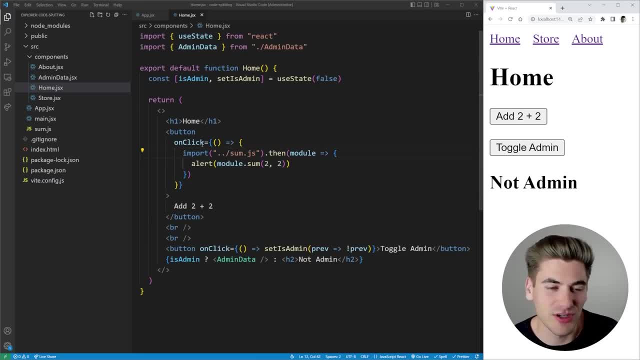 which is where code splitting comes in, And this is great for individual functions like this sum function. But where this becomes really useful is for code splitting out your different components, And react has a tool called react dot lazy which makes this incredibly easy. 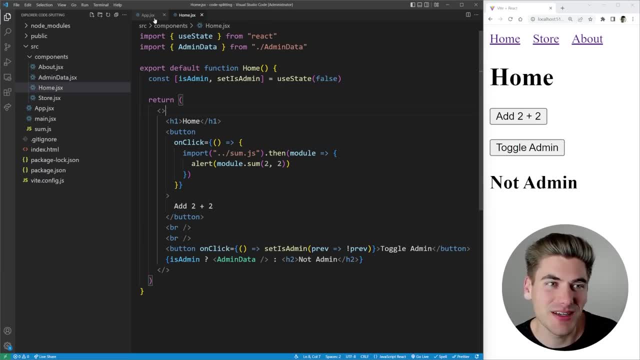 Now, probably the number one place that you're going to be wanting to do this code splitting is going to be inside of your router. Obviously, if you're on your homepage, there's no point downloading the store or the about components, And that's going to save you. 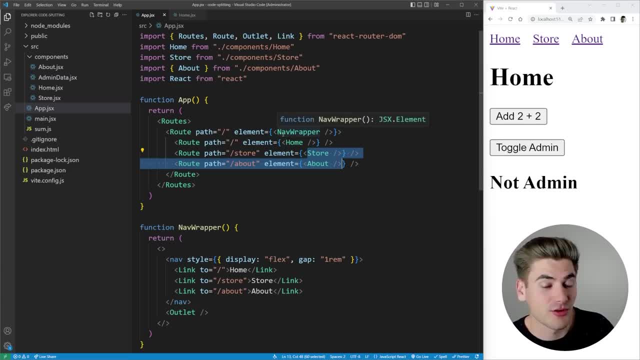 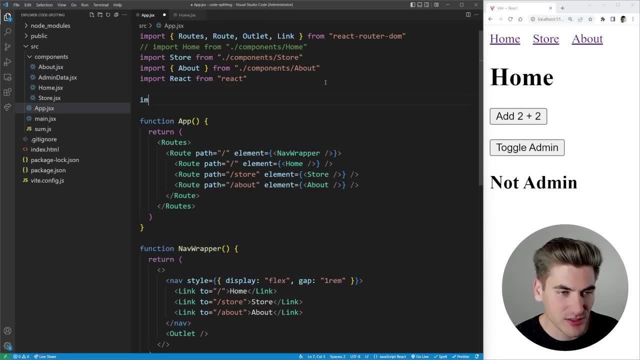 a lot of time because just downloading one page is much quicker than downloading three or hundreds or 1000s of pages. So to do this code splitting, we're going to remove our normal import statement and we need to do a dynamic import, That this is going to be an import where we call a function and we pass it in our path. 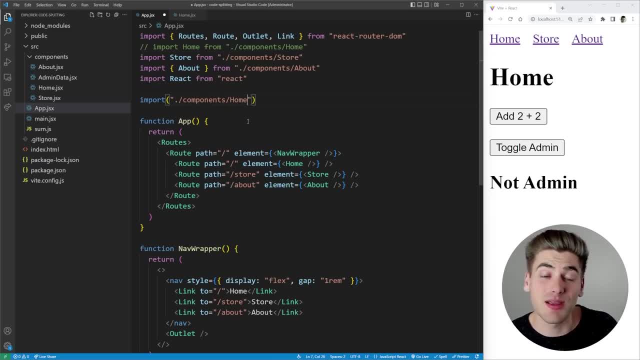 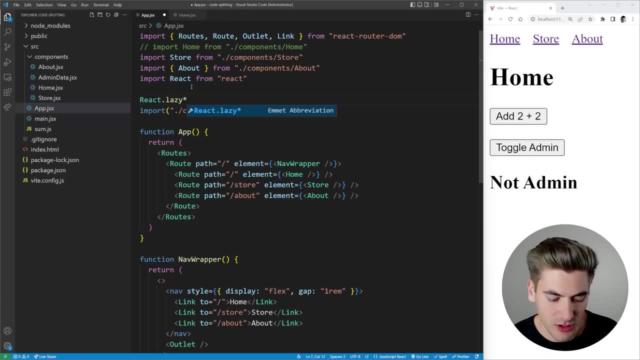 which is in our case our home file like this. But to do this with a component inside of react we need to use react dot lazy, So we can say react dot lazy. Or if you don't want to call react dot lazy like that, you can just import the lazy method up here from react And then it's. 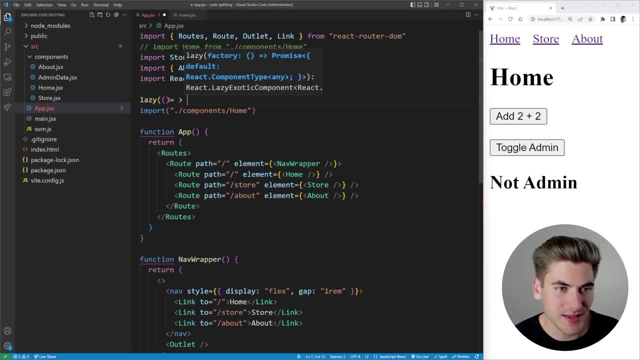 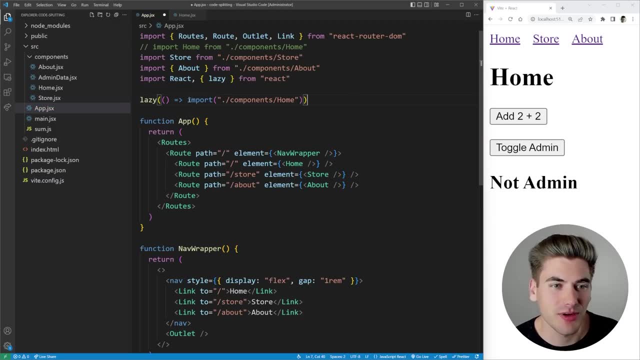 going to work just like this. So, inside of this lazy method, you pass it a function And this function, right here. all it needs to do is return a promise, which is this import statement. So we do our import. this returns the import statement, And then we're going to import the function. So 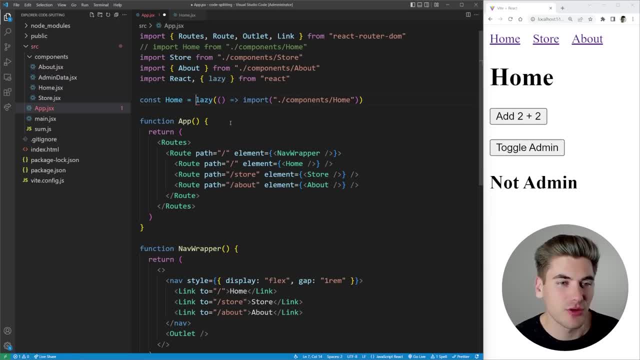 it returns to us a promise, And then this right here is going to return to us a variable we can use, exactly the same as our normal component we imported. So if I save, you'll notice. if I just do a refresh over here, everything looks exactly the same as before. And if I go to my store page. 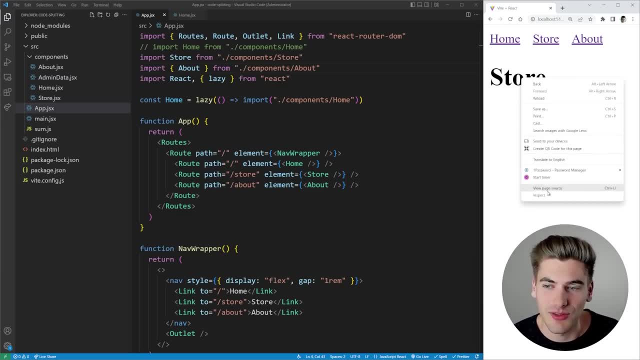 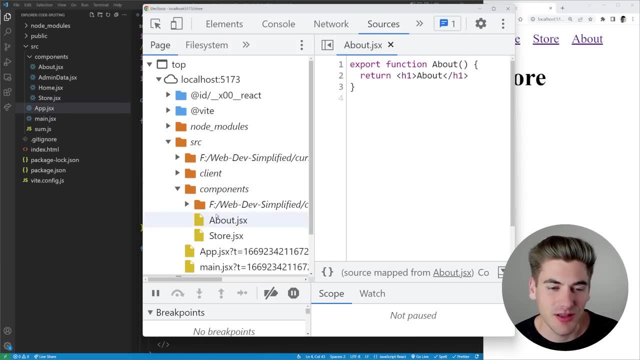 and do a refresh. that's simulating me coming to the site directly on the store page. You'll notice if I go over to that sources tab real quick. I just close that everything And we look inside of our components. the homepage component is not being downloaded yet And 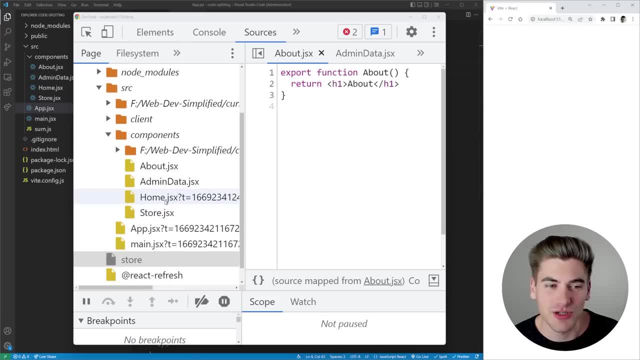 as soon as I click on that homepage button, you'll see now all the information for my homepage, including that admin data component are all being downloaded after the fact, So I'm only downloading the components when I need them. You will notice a bit of an error, though, in that. 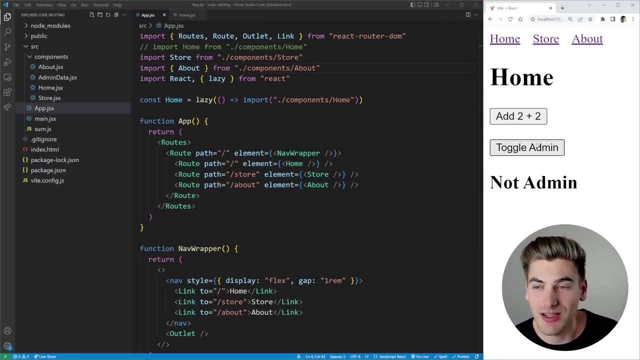 none of our content is actually showing up. If I do a refresh, you'll see the content shows up, but it's not showing up when I click on that link for the very first time. The reason for that is when you're using this lazy loading of components. React needs to know that you're lazy loading. 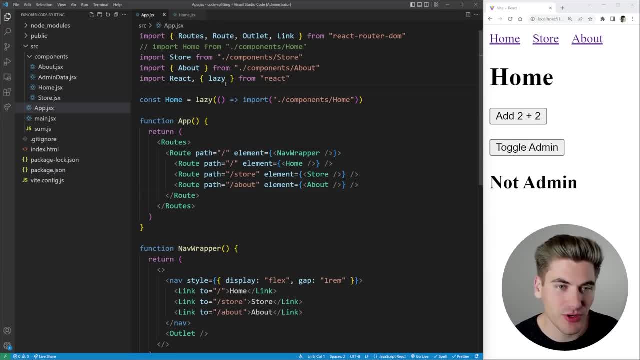 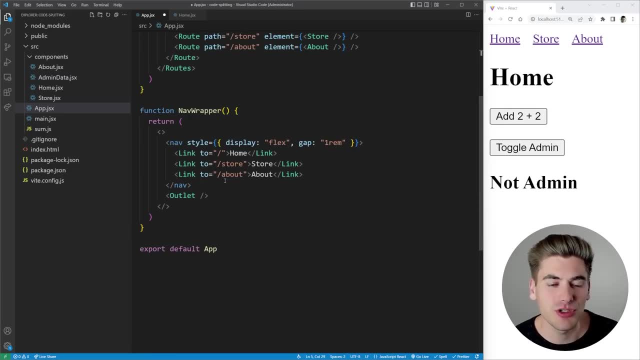 different things And you need to use suspense to do that. So we're going to be importing suspense from React And I'll show you exactly how this works and why it works like it does. So this is a fancy component inside React And what you want to do is you want to wrap whatever is going to be. 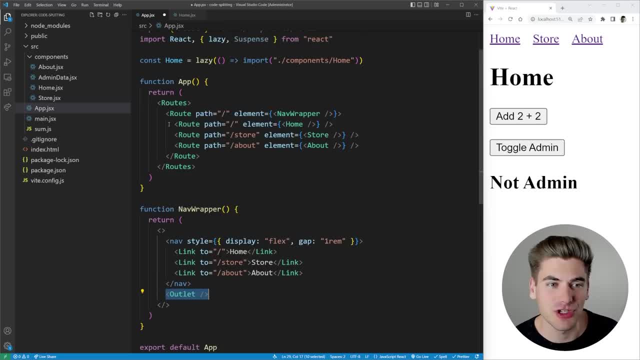 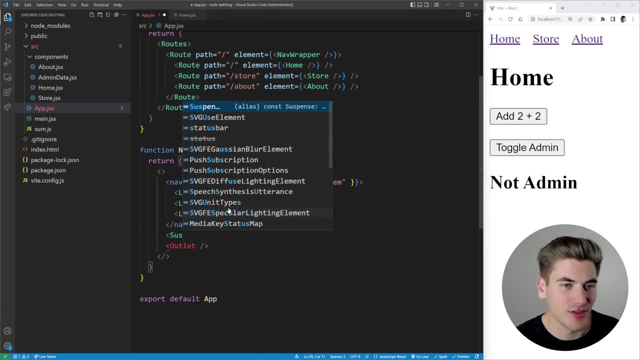 lazy, loaded inside that suspense. So this outlet right here just renders, whatever our route is, in our case, our homepage, our store page, our about page, So we can just wrap this outlet inside of this suspense component And now, if we do that we're telling: React everything inside. 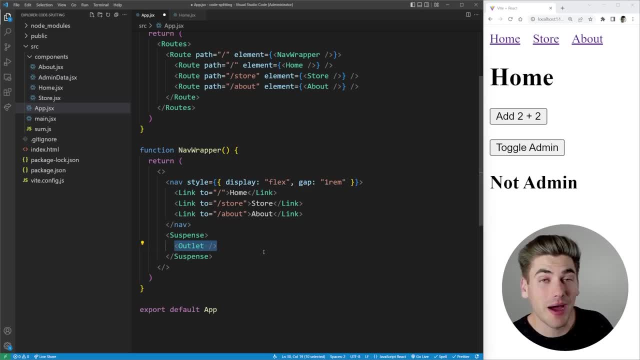 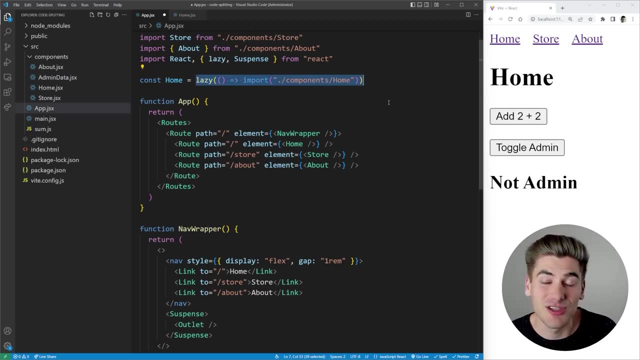 of here has the potential to be lazily loaded, which means it might not be available right away. In our case, when we click on the home link, we're going and downloading this home component and then rendering it when it's finished, So it'll. 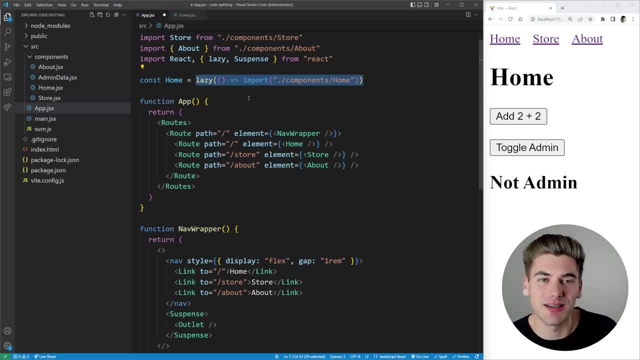 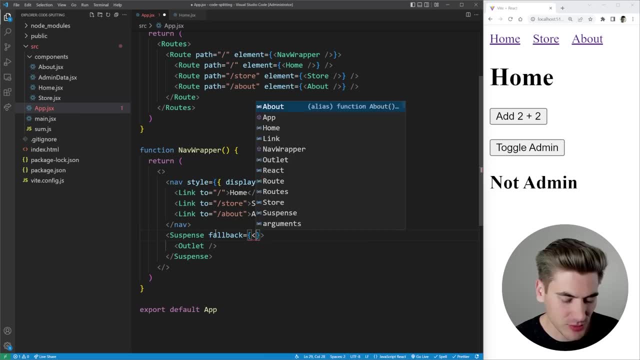 if it's a large component or maybe your internet is really slow, this might take a while, which is why the suspense component has this fallback feature And whatever you put in here, it can be a component, it can be text, whatever you want. we'll just put like an h1 that says loading. 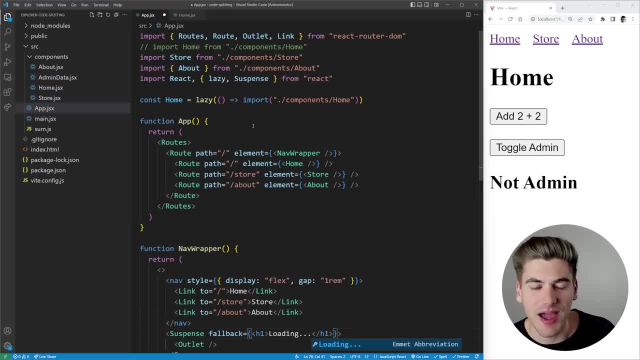 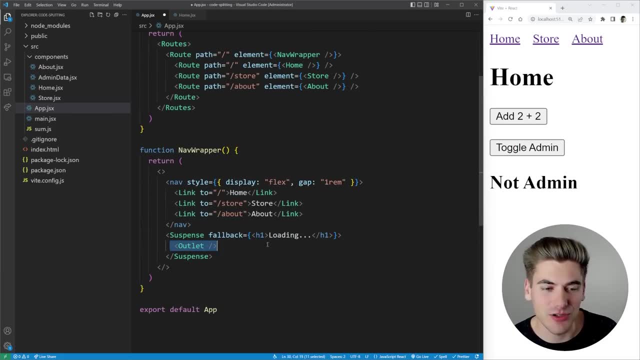 whatever you put inside of here is going to be rendered instead of the actual content. that is right here. So, while this homepage is being downloaded, it's going to say loading on the screen And then, once it's downloaded, it's going to show that normal content. So let's go over to 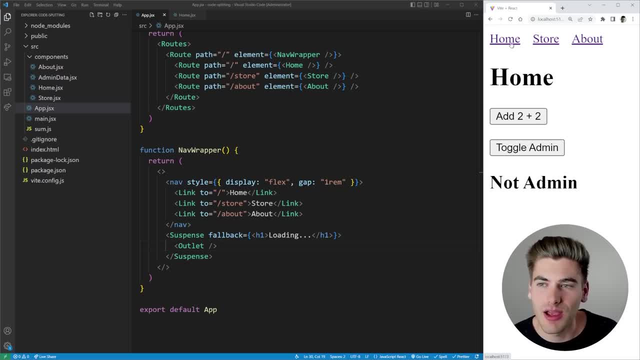 our store page. do a refresh to simulate what happens when we click on home And you'll notice it says loading dot dot dot. Now, obviously my internet is quite fast And I'm only downloading this file locally, So it's going to be incredibly quickly. But if we had a much slower loading time, 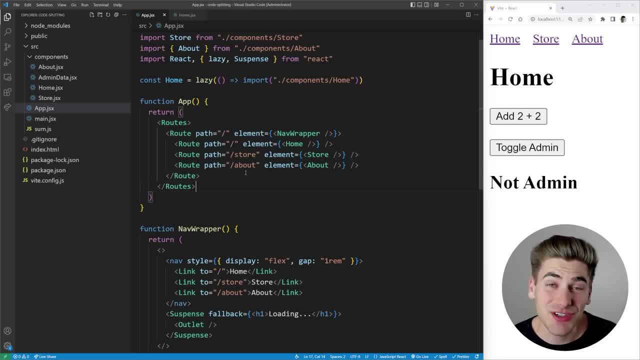 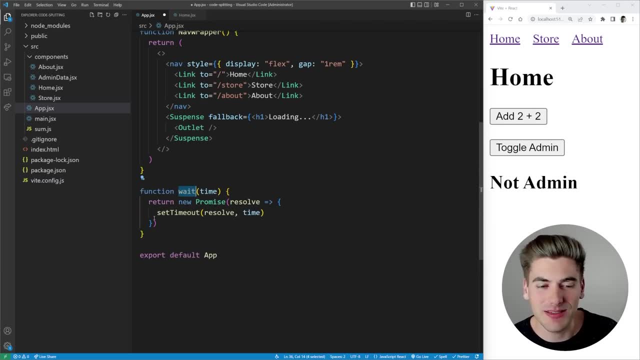 this would be a loading screen that would show for quite a while. this is actually something we can fairly easily simulate. I'm just going to really quickly create a dummy function. This function is called wait, And all it does is it waits until a set timeout is complete. So what I can do up here, 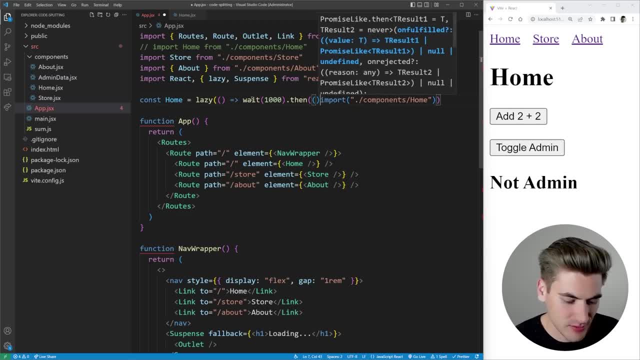 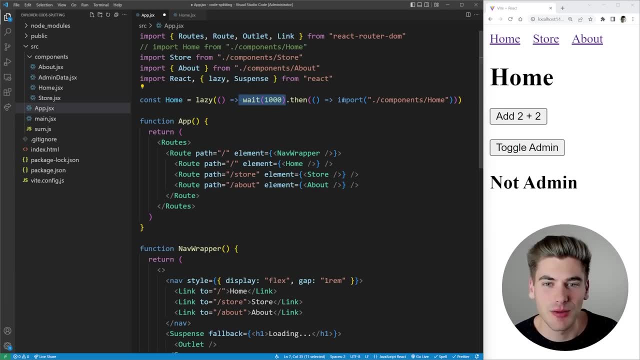 is, I can call wait with 1000 and then just say dot then and then actually return the value for this. here All this code is doing is saying wait 1000 seconds before doing my import, So it's simulating what a slow connection would look like. So now, if I just go over my store page, 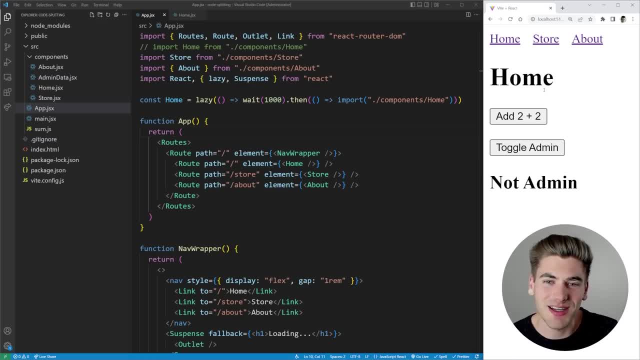 do refresh here. click on home. you'll notice it says loading for one second before my actual content shows up. So if this was a slower internet connection or maybe you downloaded a large file, you can kind of see what that would look like. And that's what this wait function is just simulating. 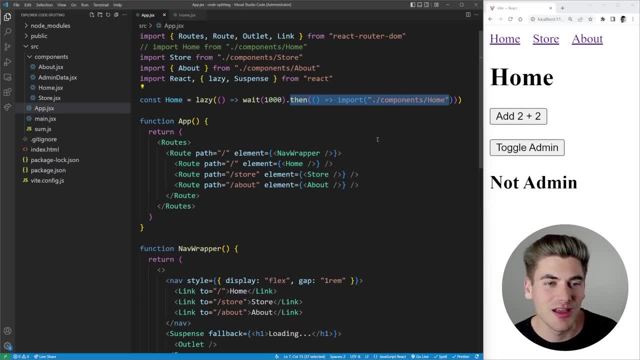 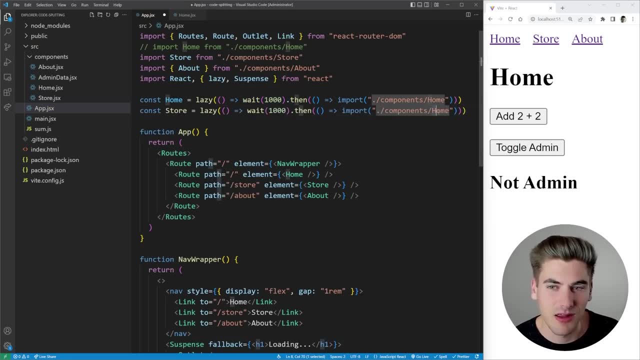 So it shows the fallback and then it shows the content once it's downloaded. Now doing this for our store page is going to be the exact same process. I'm just going to copy this all down. We're going to say store right here And we're going to import that from store, just like that. 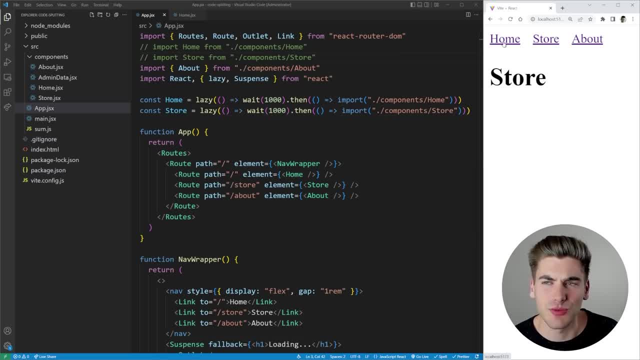 And we're going to comment this out, And you'll notice that switching between these views works exactly the same. And something else that you'll notice is when I go back to my store page, you'll see that there's no loading. that happens. same thing back to home. The reason for that is: I've 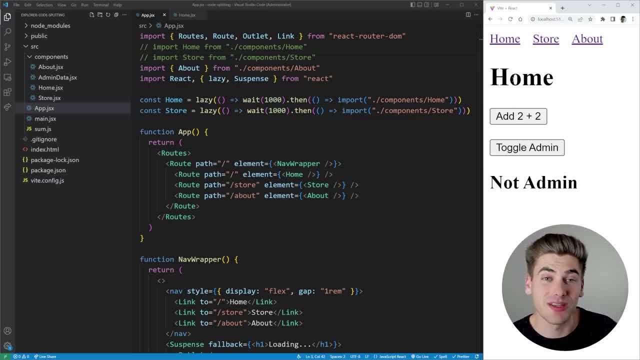 already downloaded that component into my browser, So it doesn't need to read: download it once. you download it once, it doesn't need to download any more times. Now we will run into a problem when we get to this about component, though. if we just copy this down, I paste in about here: change this to: 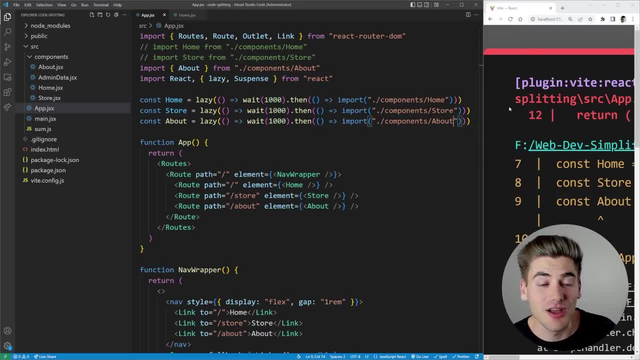 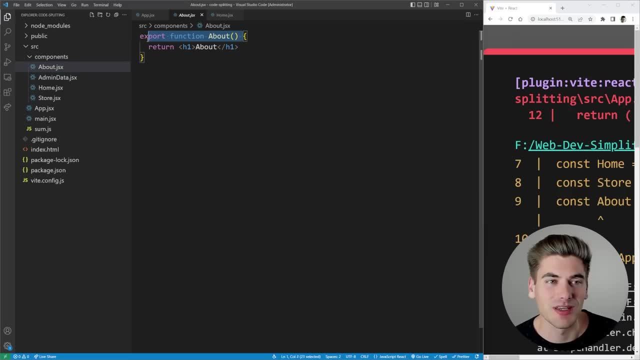 a save, you're going to notice, boom, we're automatically getting a bunch of errors. The reason for that is, if we look at my home component, my store component, they're exporting default functions, while my about component is exporting a named function. 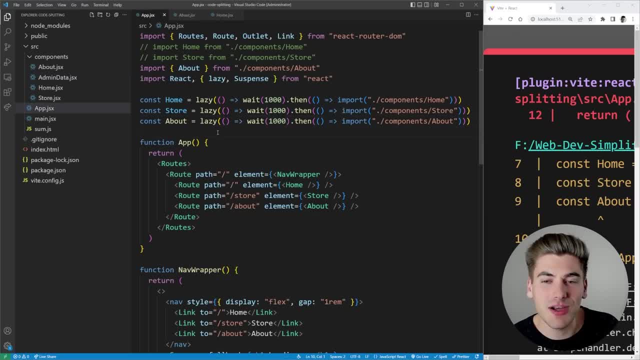 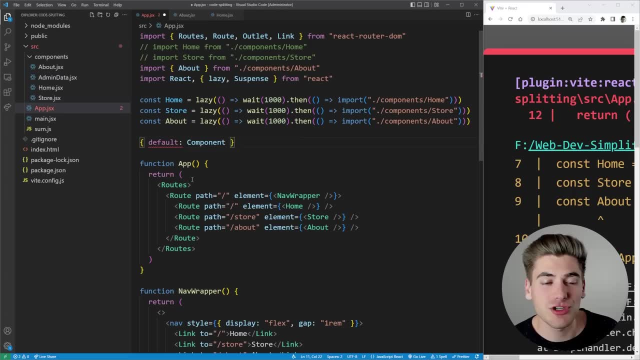 And the way that this lazy import works is it expects you to return something that looks like this, where it has a default, and then this is going to be, you know, your component. So it expects you to return an object that has a default property, and then it has an. 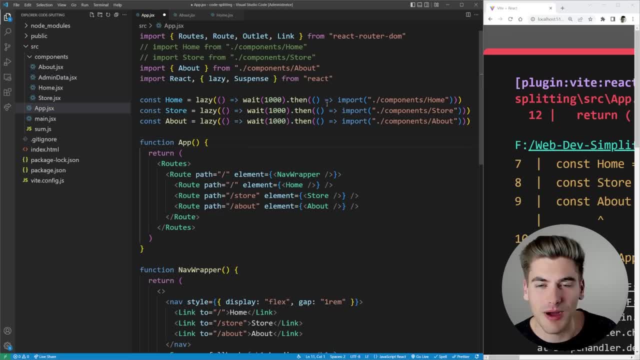 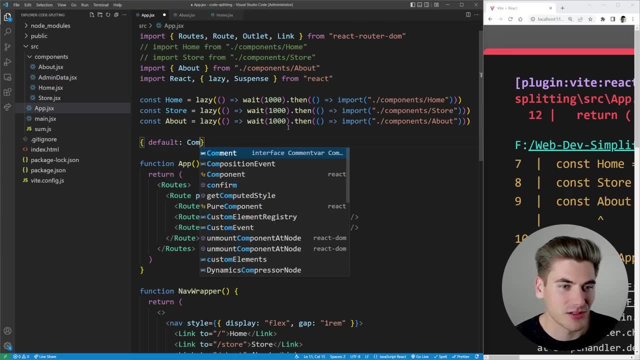 actual component in that property. So with all of our normal module imports, that works just fine, because when you do a dynamic import you're going to get a return that looks like this: So, for example, you have your default and that's going to be your component. 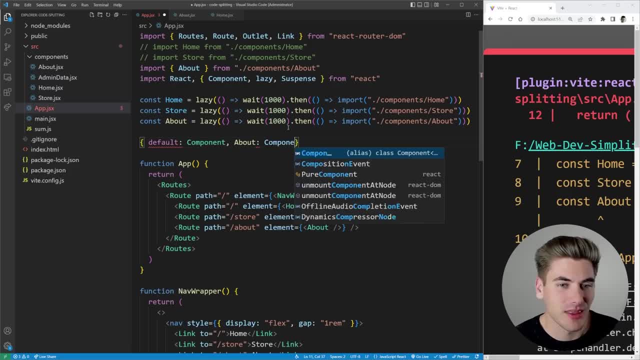 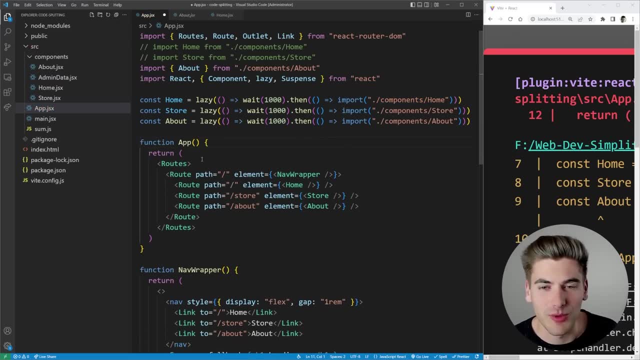 And then if you have a named export, like about it's going to be, you know something that looks like this. So by default, all of these that have default exports are going to work just fine, But our named exports don't work quite like we would expect. 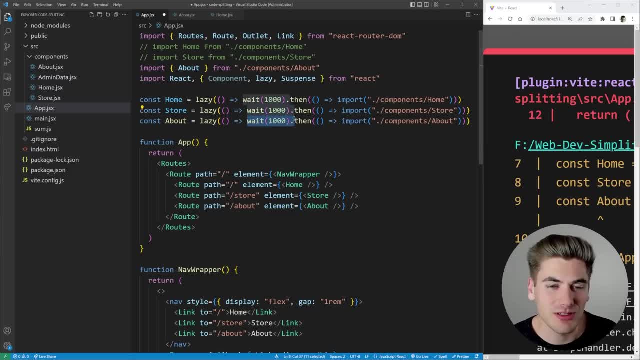 So, in order to fix that, we can do a little bit of tweaking. What I'm going to do is I'm just going to remove this, So it's a little bit easier to read what's going on, get this back to just a really simple, normal import Whoops. there we go, And what I want to do is I just want to. 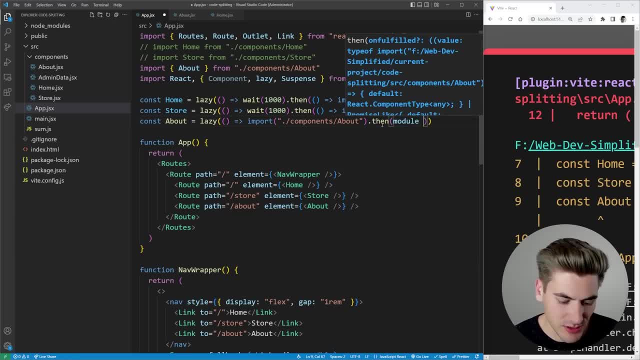 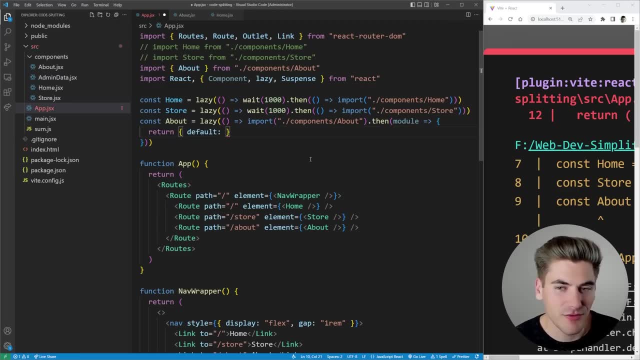 say dot then and I want to actually get my module that's being returned to me And my module here, like I mentioned, has that about property. So we can say we want to return a property, that is default And we're just going to set that to our module. dot about. 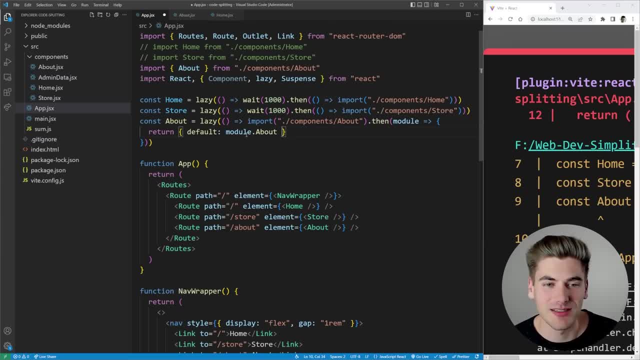 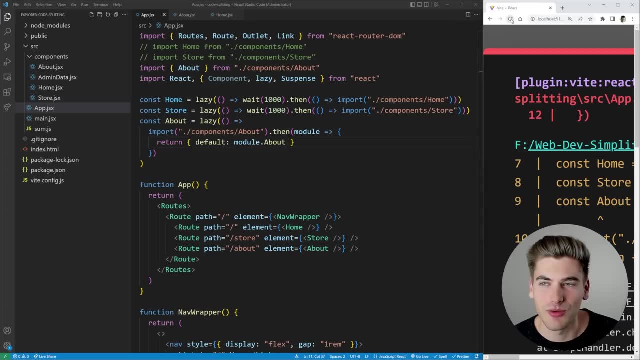 all that this is doing is essentially renaming our import so that, instead of being at dot about it's at that dot default And that little change, right there is all we need to do to make this work. We just give this a quick refresh here. you notice it's still not quite working. That's. 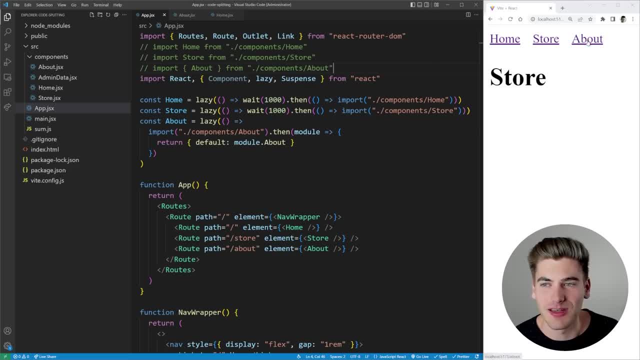 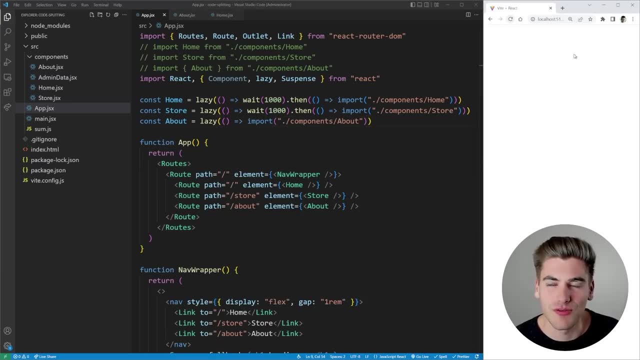 because I forgot to comment this section out up here. Now, if I save, you'll notice that it is working just fine when we go to that about page- And just to prove that it wasn't working before, I'll remove all the code I added. click Save, do a refresh and you'll see that the about page 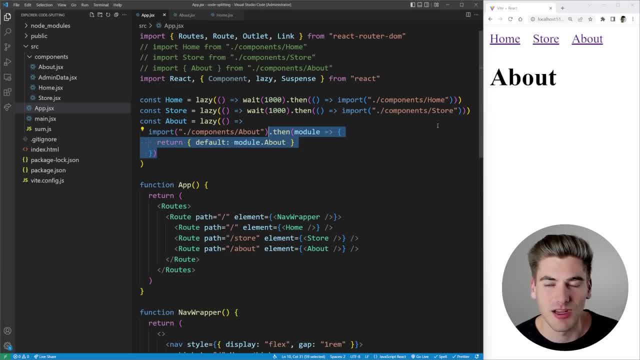 doesn't show up. So there is an error if we don't do it like we expected. Now, if we put it back, you can see that it works. Now this may be the most common way that you would do code splitting by doing it based on your pages, But a lot of times you may have content on your page which 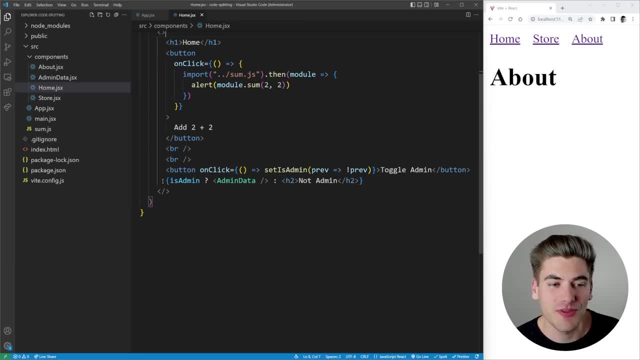 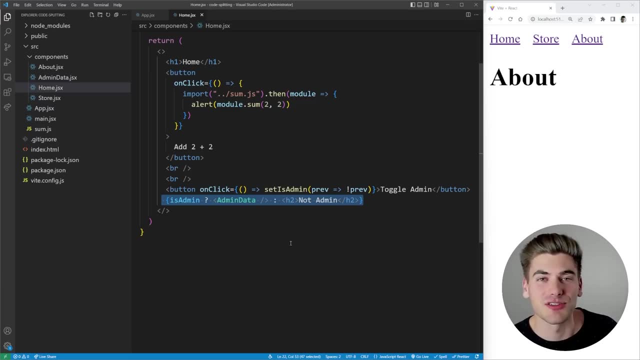 is only applicable to certain users. For example, on our homepage we have this section for our admin data, And imagine this is like a crazy big admin dashboard that shows up for admin users And for users it doesn't show up. So it's a very large amount of data that's being downloaded. Well, 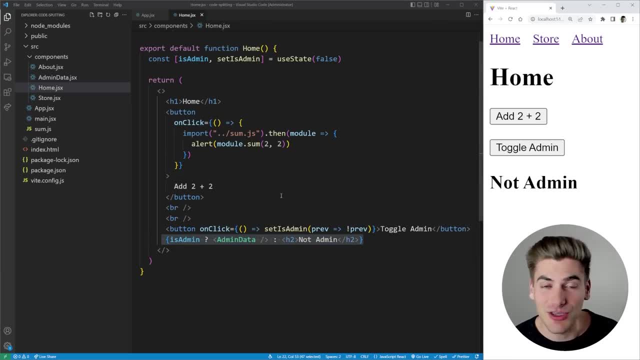 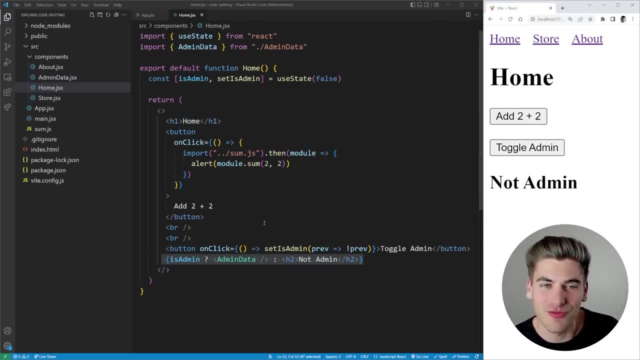 you wouldn't want to show all of that data every single time any user went on the page, even if they don't have access to it. there's no need to download that information. So we can again use code splitting to make sure we only show that information if this person is an admin. 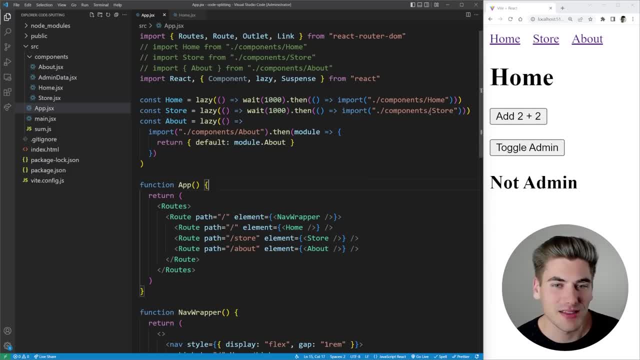 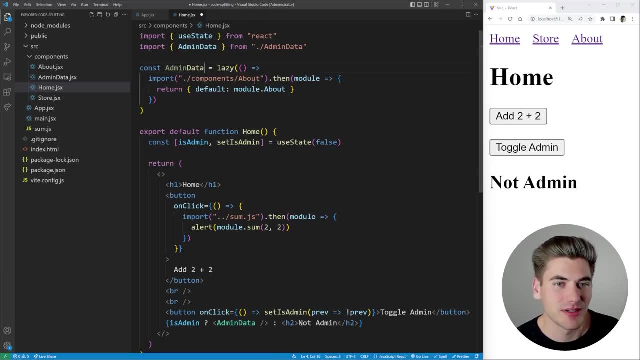 So instead of doing our normal import like this, let's do it the React lazy way. So I'm just going to copy over this code exactly from our about here and paste it down, because this is a named export, So we're going to call it admin data. It's coming from our admin data. 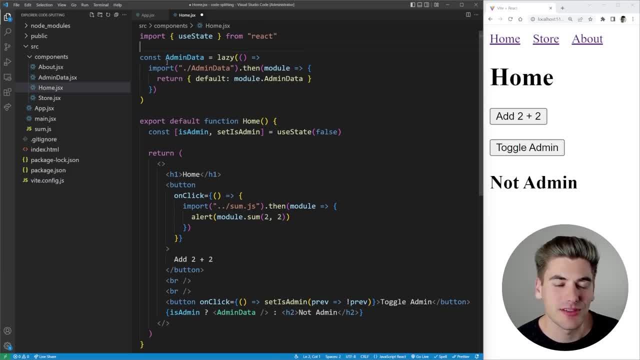 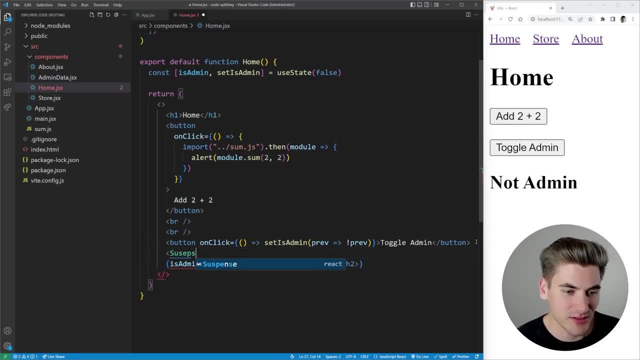 component And here we're getting our admin data. that, right there, gives us the admin data itself And it's being lazy loaded. all we need to do is wrap this inside of a suspense. So here we can say: suspense, Just like that. Give it a fallback. Oops, fallback is equal to. let's just say: 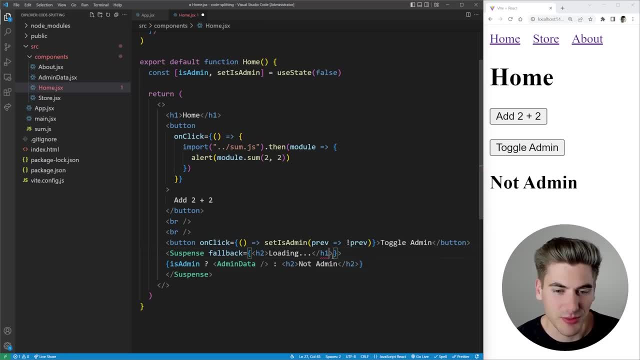 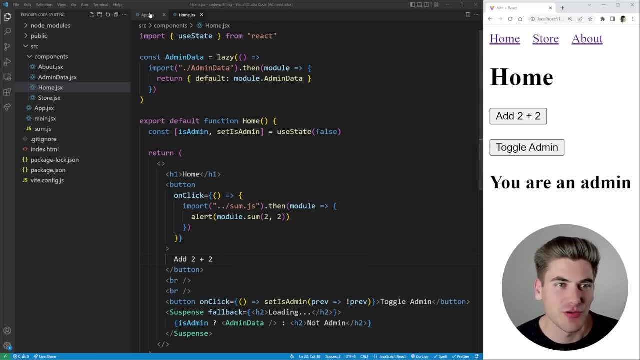 loading. Let's make that an h2 just so it matches up with the other content in that section. And now if I give this a quick save and I click type we'll admin, you should see it would show the loading text. But this is way too fast. 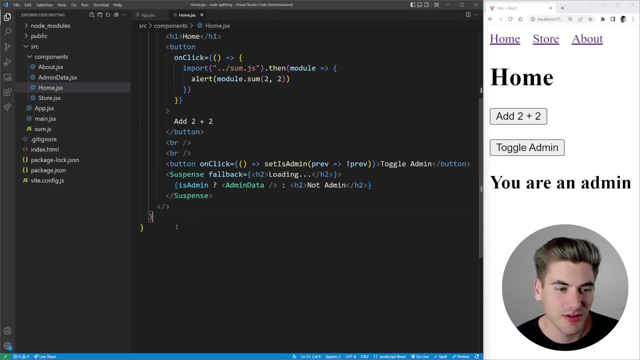 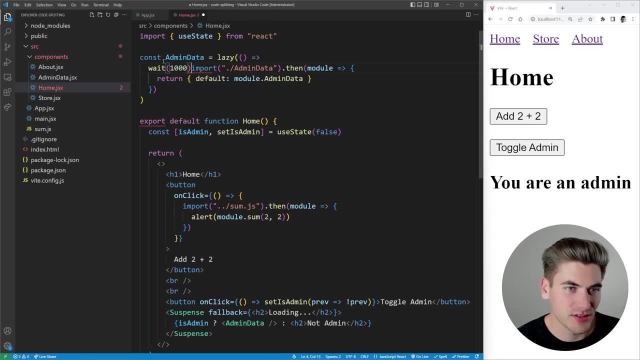 Let's slow it down with that artificial wait, just so we can see what would happen. So I'm going to paste that function down And up here. I'm just going to do a simple wait dot or wait for 1000.. So that's one second And then we're going to call this import right here. 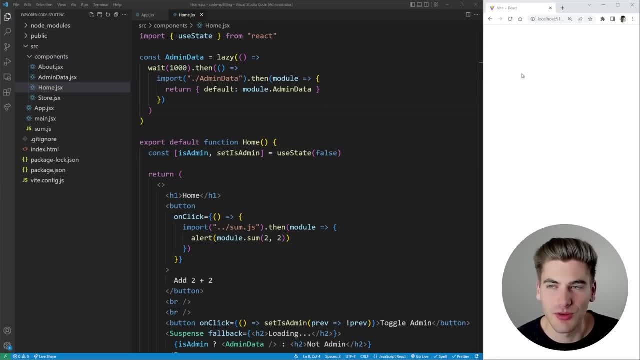 There we go. So now let's just do a quick refresh. you can see it's loading my homepage and we're getting an error. The reason is is we need to make sure that we import lazy and suspense, So let's just import both of those. 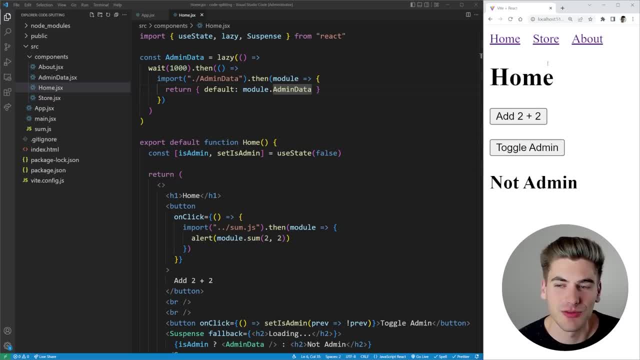 And now, hopefully, if we give this a refresh, it should work. And there we go. you can see it's working. Now, when I click toggle admin, that's going to make my admin true, which means we're going to show this admin data which is being lazy loaded, So it should show us the text loading. 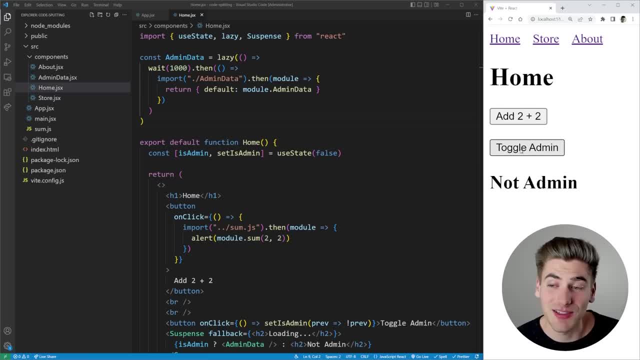 As you can see, it shows the text loading and then it says you are an admin, And now I can toggle between the two with no problem. So if you're a non admin user, it's never going to download this content because it doesn't need it, But if you are an admin user, it'll download it. 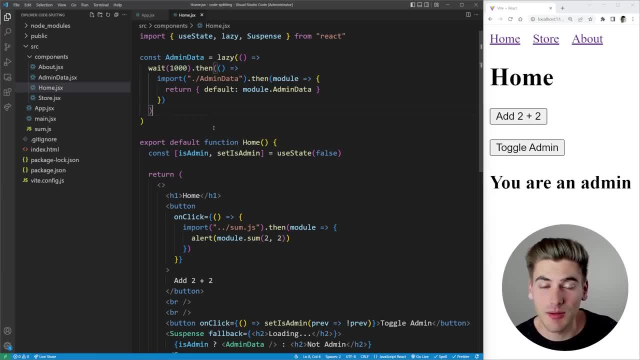 when the page loads and it'll give you a loading bar. Now, the last thing I want to talk about when it comes to lazy loading is what happens when you don't actually want to show a fallback State. So, for example, normally we have this loading text that shows up when we change between. 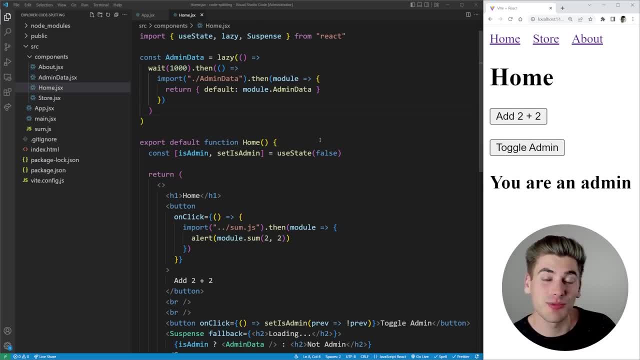 these things. But what happens if you have like tabs on a system and you want to just keep the old data there until the new data is finished loading? This is a fairly common use case. Well, to do that in react, we need to use the use transition hook. Now, this is a hook that I have. 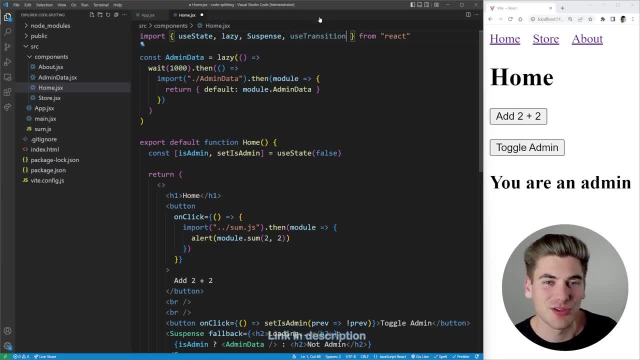 an entire video on. I have an entire course action, all the hooks. I'll link it down in the description for you if you want to learn more about how this hook works. But essentially it allows us to do non urgent updates which won't change our UI until they're finished updating. So what we can do. 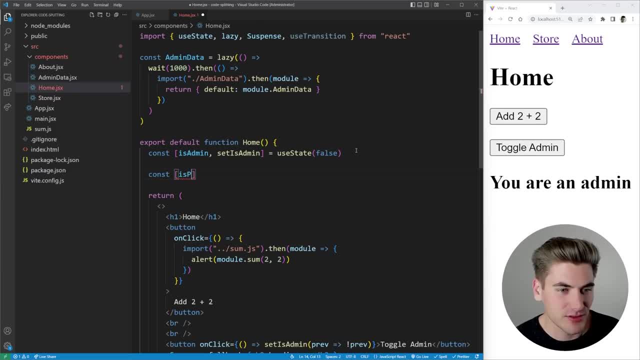 is, we can just make sure we call that hook And then we're going to go ahead and hit save And that hook is going to return to us two values. The first is going to be: is pending, which we don't actually care about, And then we can have a start transition, which is the thing that we 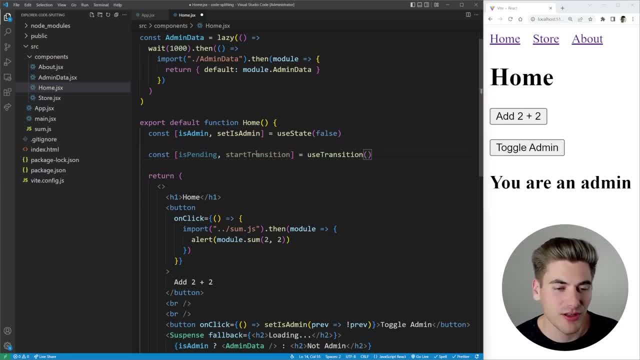 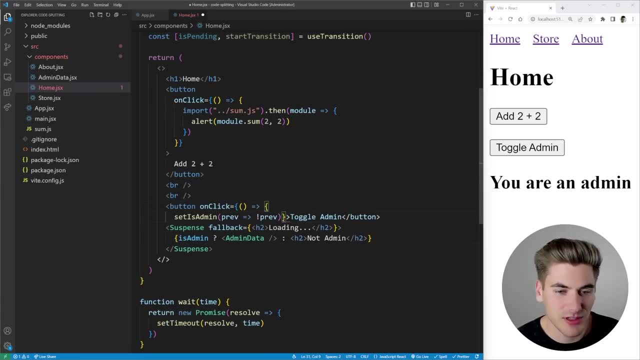 care about, because that allows us to do this update. just call that hook, there we go. And now what I want to do is, when I click on this button here to set is admin instead. I want to put that inside of a transition, So I'm going to bring this onto a new line just to make it easier. 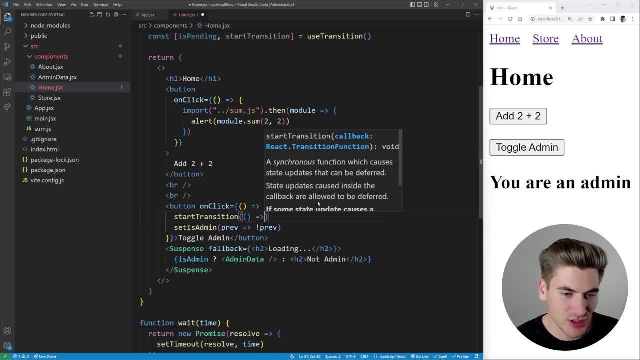 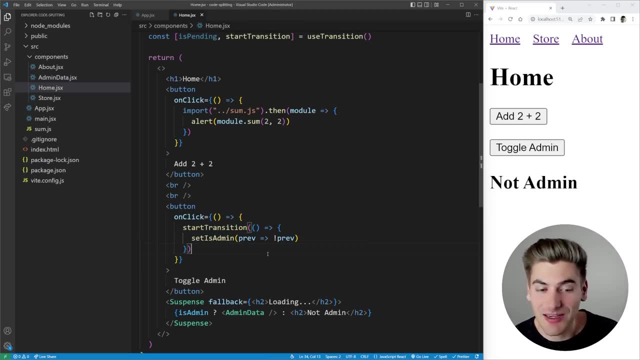 to read. I'm going to call start transition And this just takes a single function And inside of here is where we put our updating for our state. So now what's going to happen is my actual UI is not going to do this fallback value because my UI is not going to update until this transition is. 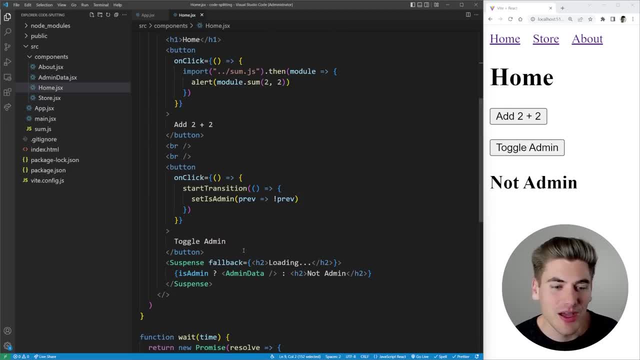 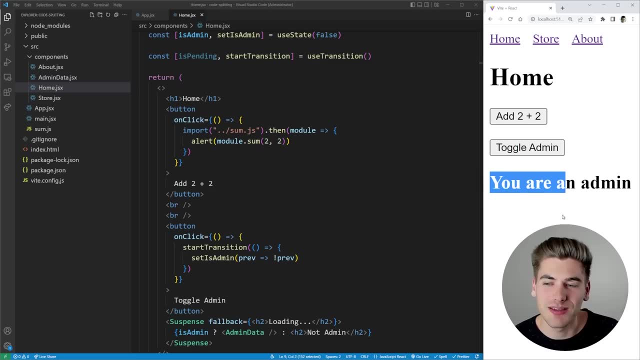 finished, which means it's going to wait for this entire thing to download before it tries to show any data at all. So when I click toggle, we'll just do a refresh First. when I click on this toggle button, you'll notice my UI doesn't change until after everything's loaded. So I don't get. 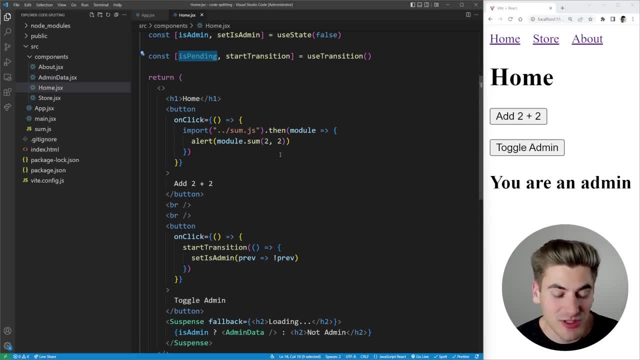 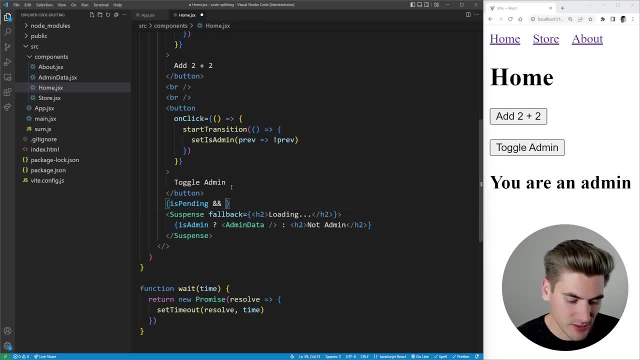 that loading state. But I can use this is pending variable to show some type of loading state if I wanted to. For example, I could just say is pending, And what I could do is I could just say loading. really straightforward stuff like that. So now let's just give this quick refresh. 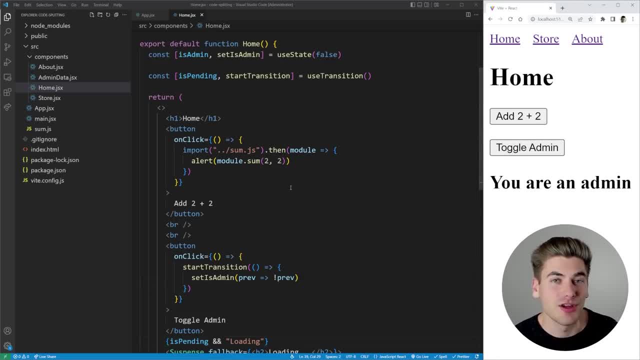 and click toggle admin, you can see it saying loading, and then it shows up right there. you could use this, for example, to like blur out the background and show like a giant loading spinner over top of everything, If you want it. that's a much cleaner way than just blanking out. 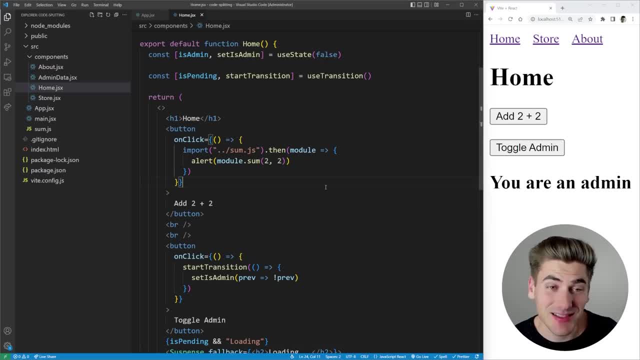 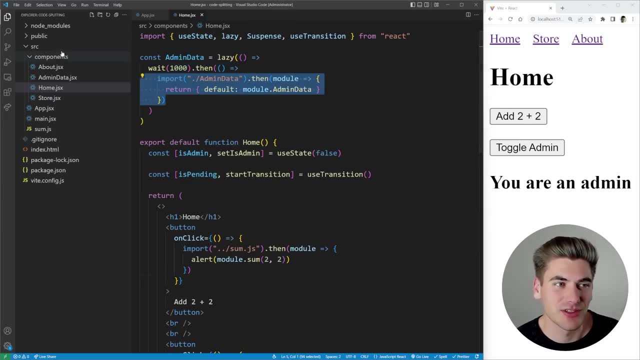 everything and showing like the text loading, for example. Now, the very last thing I actually want to talk about is if you're doing a lot of deep or named exports like this. it's kind of cumbersome to write out your imports like this every single time, So actually I recommend just creating like 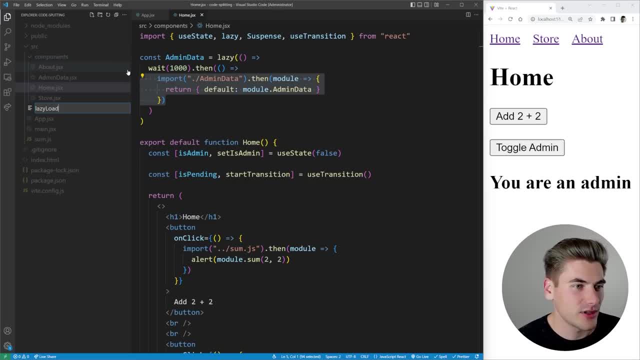 a really simple function. we'll just call this lazy Load dot j s. let's paste the code in here. Essentially, all this code does right here we'll get rid of the weight, because that's not actually part of it. 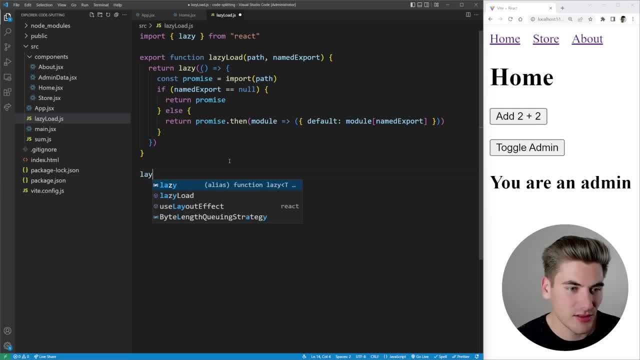 All this code is doing is it's making it so you can call lazy load, you can pass it the path to your component. for example, let's say slash components, slash about, and then we can say that this is an about named component. this is going to allow you to import something that has 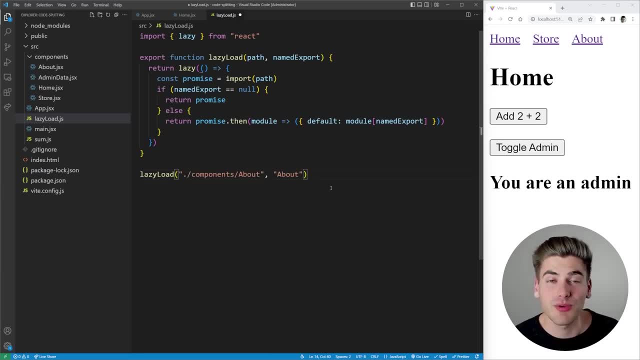 the name of about from this actual URL, And that's really great If you don't use default exports. I almost always use named exports like this, So having this little handy function makes importing these things with react dot lazy a lot easier. As you can see, the code just calls that lazy. 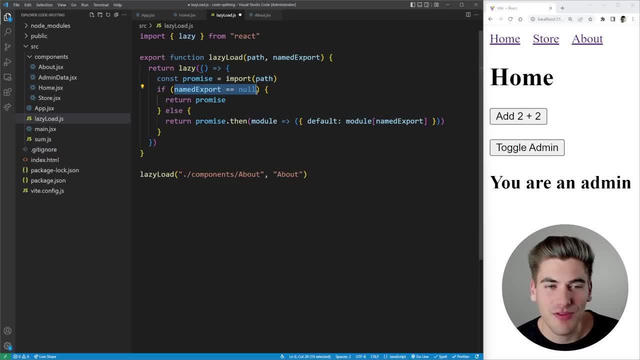 function for react. it gets a promise for my import if we have the named path. So, for example, if you don't pass in a path, it just gives you the default export, like normal. Otherwise, if you do pass in a path, what it's going to do is just going to take that path name and set it as the.